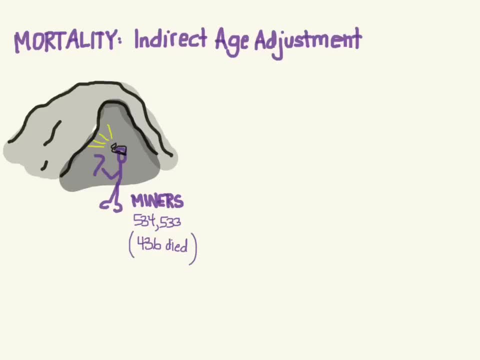 And so you're starting to wonder: is there something in the mine that's killing these people? Is this 436 consistent with the death rate of the town? Is this 436 consistent with the death rate of the town in which they live? So our question is: is this death rate here the same death rate as we're seeing in town? 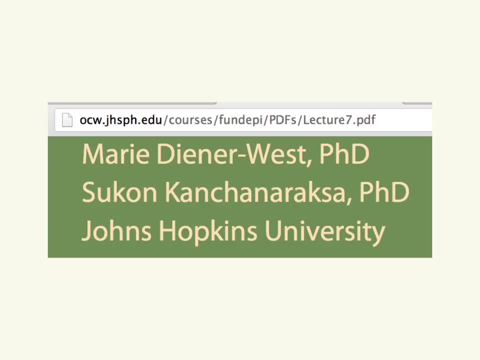 And so this example again comes from this same presentation that I used in the previous example, which the website is here. It's under Creative Commons license, And I want to make sure we give credit to these nice folk here who came up with this data set. 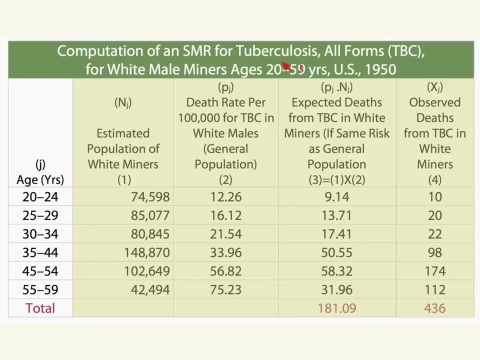 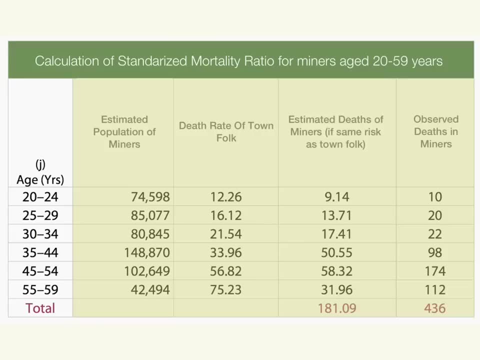 And the actual data set looks at tuberculosis in white. There are white miners in this town, but I simplified it a bit And we're just going to look at the death rate, not necessarily death rate from tuberculosis, but death rate of these people. 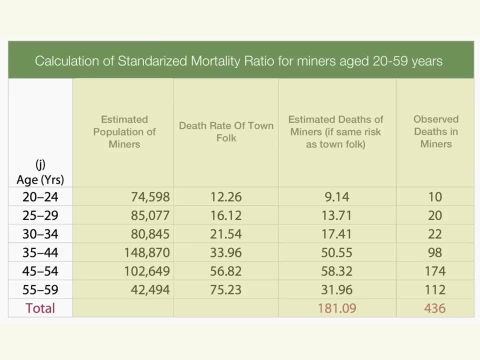 And I changed it to town folk and miners so we can see. So what we have here- so let's go through this In the first column- is our estimated population of the miners, And so we can see here how many miners we have. 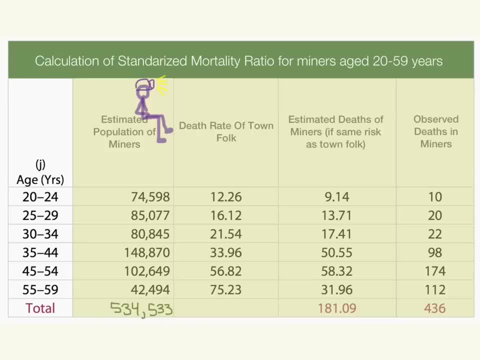 We said the total number of miners was about 500,000 over here, And in this column we have the deaths of the miners. Before we go there, let's look at this. So in this column we have the death rate of the town folk. 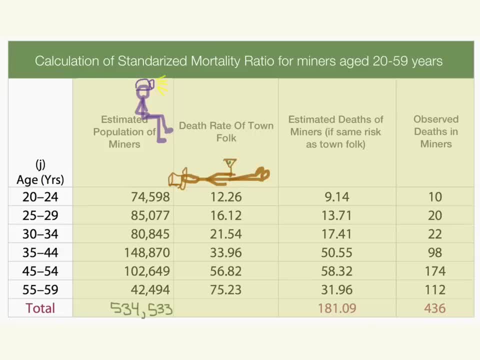 And so here's a dead townie. Look, he didn't even spill his drink. And so for this group, for the town folk, we do have age-specific mortality rates, And we have that here, And I should say that these rates are. 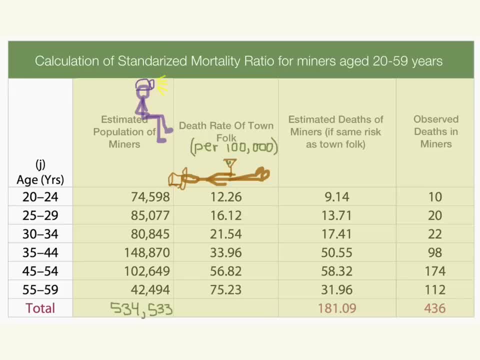 Per 100,000.. So what we're going to do next is we're going to apply the death rates of this population- the townies- to the miners and say, all right, if we use this as the standard population, and we're going to use the miners as the standard population and use this death rate. 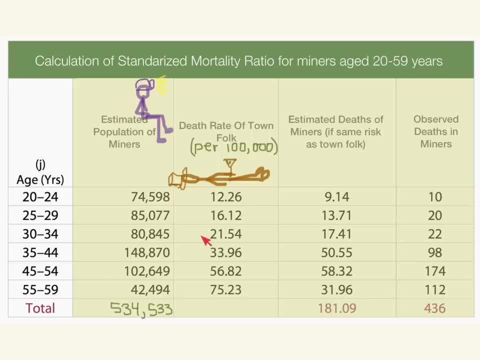 how many dead miners would we expect to see if they followed the same death rates as the townies? And so we would multiply 12.26 divided by 100,000, right Times this population. So we would say 12.26 divided by 100,000 times 74,598. 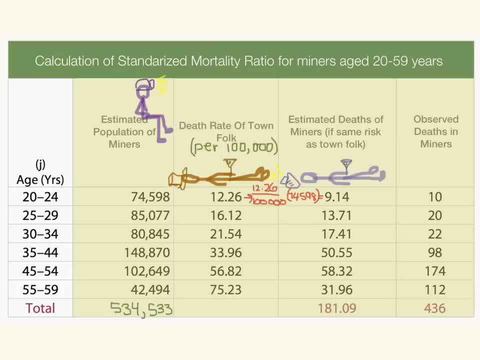 We would get 9.14.. So if the miners died at the same rate as the townies did- See look, he's even got a drink too- Then you would expect to see 9.14 deaths in this age group. 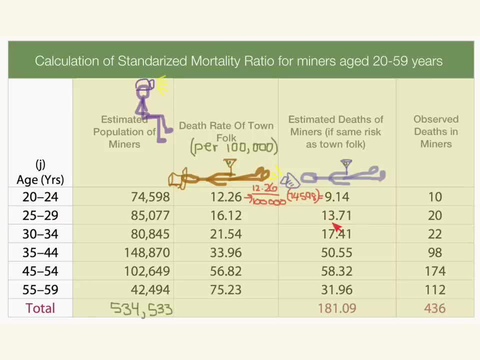 In the next age group you'd see 13.4.. In the next age group you'd see 13.71. And so on and so on down the age groups. you would see this. Now we can actually see how many miners actually did die. 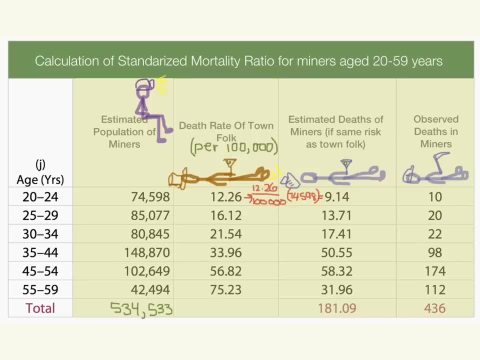 And take the real numbers, So this is the real number of miner deaths. So he has his X or whatever the heck it is that miners use, And these are the real numbers we observed, So we can add these up And so we have the estimated. 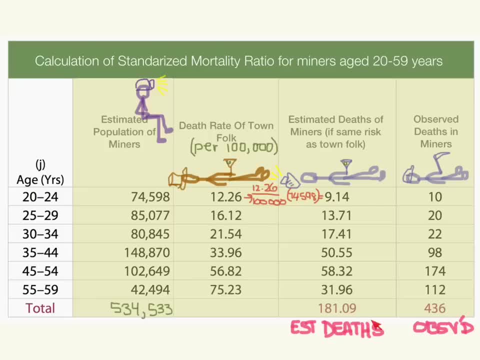 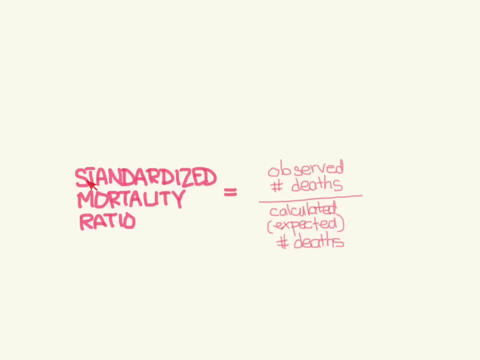 The number of deaths and the observed number of deaths. And now what we can calculate is called the standardized mortality ratio. And so what the SMR, or standardized mortality ratio, is? it's the observed number of deaths over the calculated or expected number of deaths. 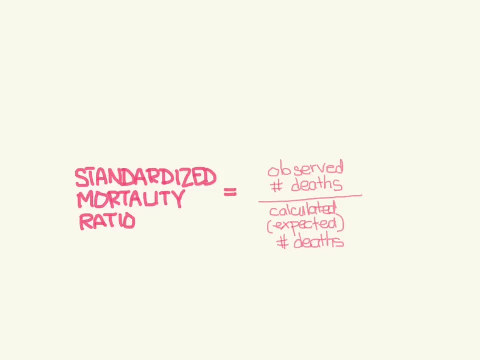 And so using the numbers that we have from the prior example, And so we had seen 436 deaths in the miners, But we had calculated 181.. And if you do the math, this comes out to 2.41 or 241%. 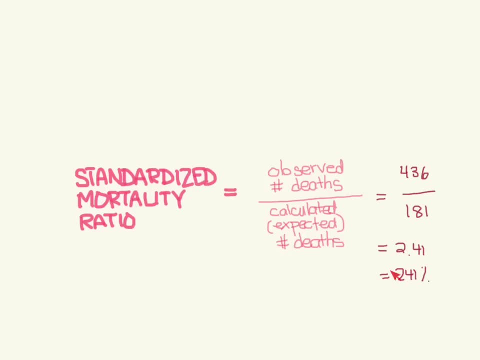 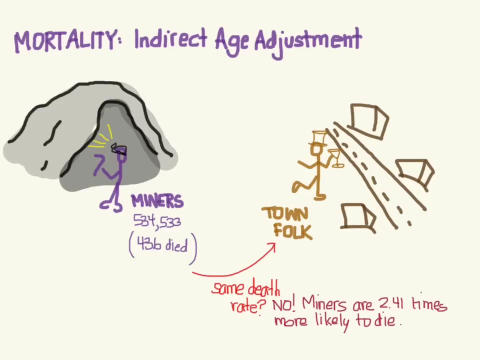 So what this means is that the miners are 241 times more likely to die than the townies are. Actually, I just misspoke Not 241.. It's 2.41.. It's 2.41 times more likely to die. 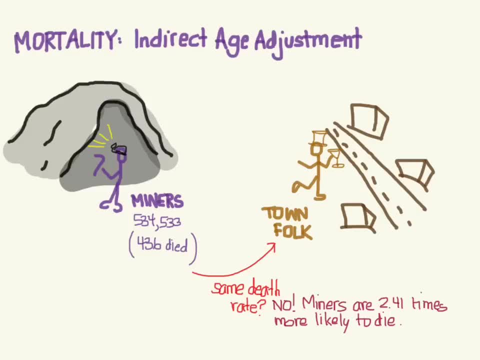 So the miners are almost 2.5 times more likely to die than the town folk are. So this number here is our SMR. So let's say that the town folk- we know that their crude mortality was 10.9 per 1,000.